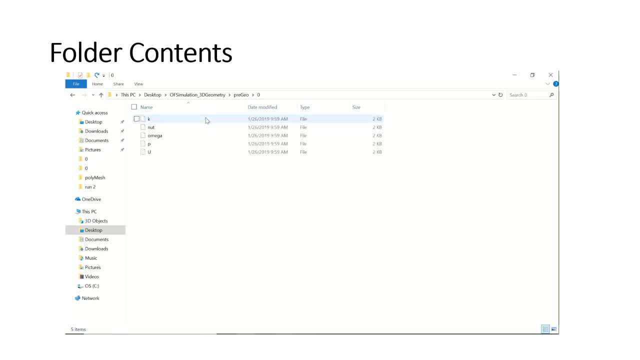 the initial condition files that go with that model are K, NUT, OMEGA P and U. In addition, in this folder we have our system and this has our FV solution, FV schemes, and that helps us with convergence. 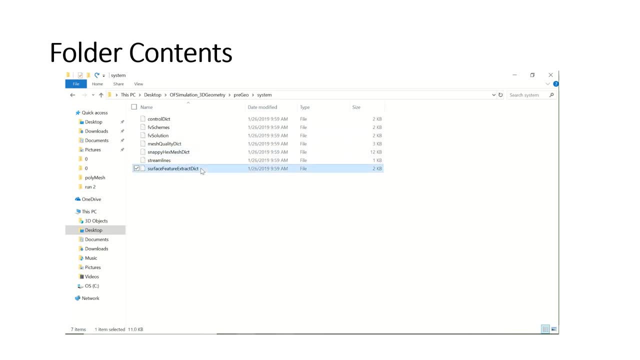 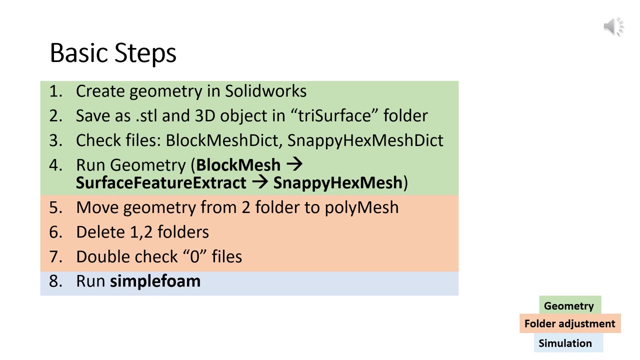 And then we also have snappy-hex, mesh dict and surface feature extract dict. So these are really important for when we actually import our STL file, when we want to run our simulation on that. So there's some basic steps to today's tutorial. First, the category in green, those steps. 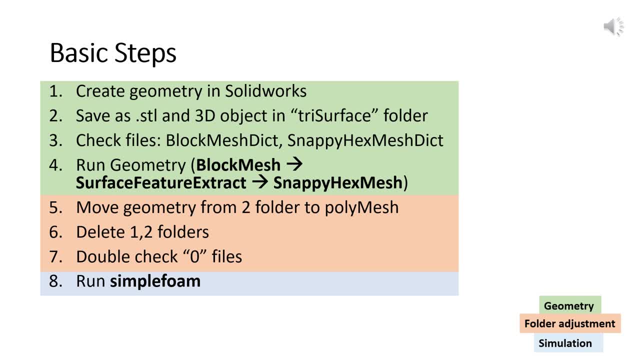 are all involving making our geometry, putting it in the right folder and then finally actually running the geometry using the OpenFOAM Simulation 3D Geometry. Then the red category. that's more about moving some of our geometry around into different folders within our actual file explorer. We have to delete a couple files after that step. 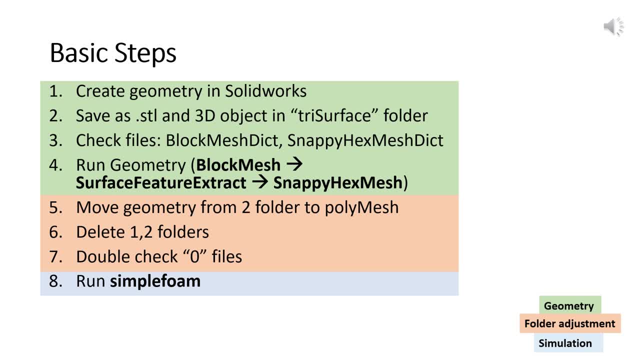 And then we'll check our initial conditions. And then, finally, the category in blue, which is just one step. it's step 8, it's actually running our simulation. So that's what we're going to be doing very last, and then we'll look at our results. 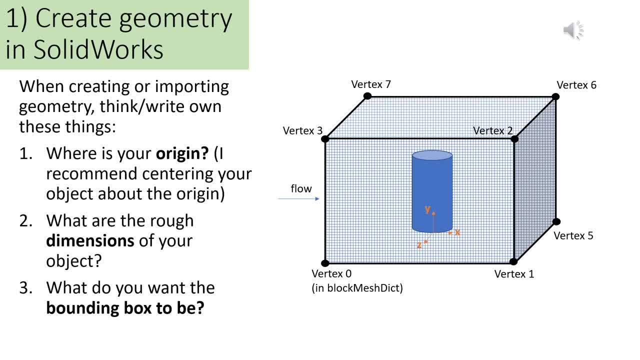 So real quick, just to make sure that you guys can see the screen. So we're going to try to get through the video. So there's a couple things you want to think about before you make your 3D geometry. is you want to keep an eye on where your origin is, both in SolidWorks and then what it's? 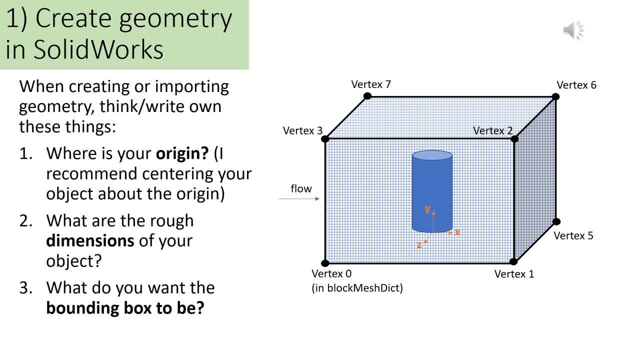 going to be in paraform. You want to think about where your block mesh is going to be around your object and that'll help you come up with where you want your vertices to be. And finally, you don't want to make your block mesh too small. The ratio between the cross. 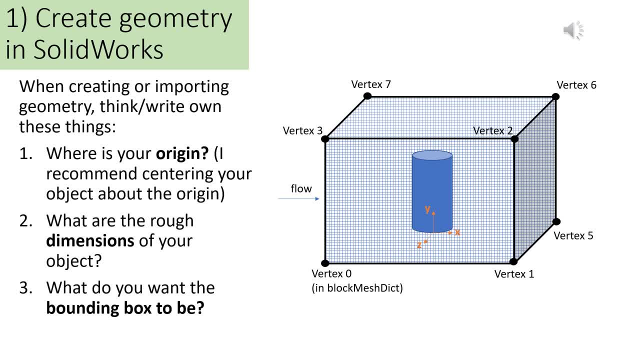 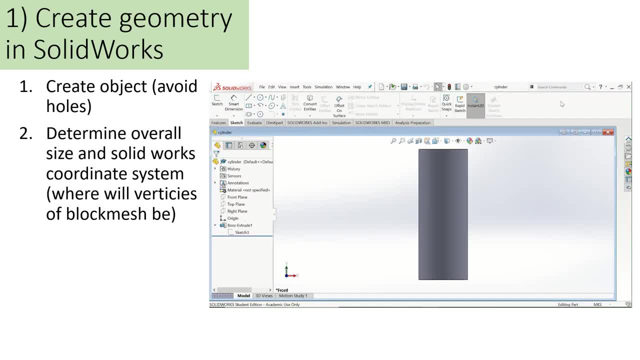 sectional area of your object to the block mesh should be about one 10th. So those are steps that you should keep in mind. Alright, so this is the geometry that's already in that folder, so you'll notice that we're in meters just because it. 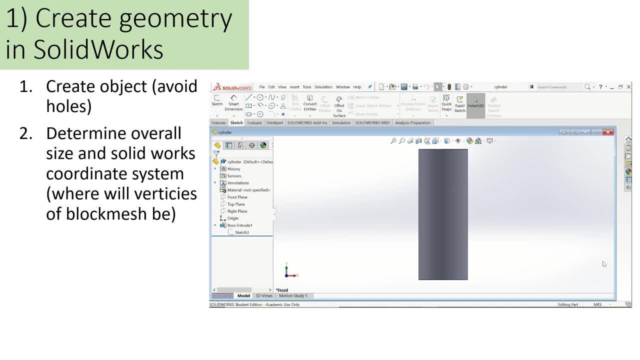 makes it easier when you're making your block mesh. A couple things to keep in mind. you're welcome to make your own geometry to import into this tutorial. you just want to keep it a couple little hints. one of them is make sure your object centered about the origin. it'll make it way easier when you have to. 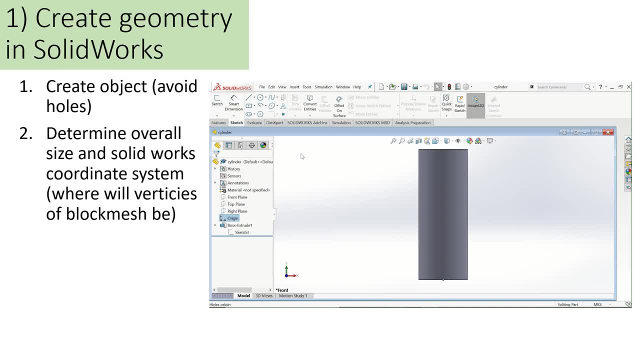 adjust your block mesh. Another thing is just keep track of your dimensions. it's really simple, but it can lead to big problems if you don't keep track of how big this is in respect to your block mesh. And then, finally, just try to keep an idea of where your inlet flow is going to be coming from. You can use this. 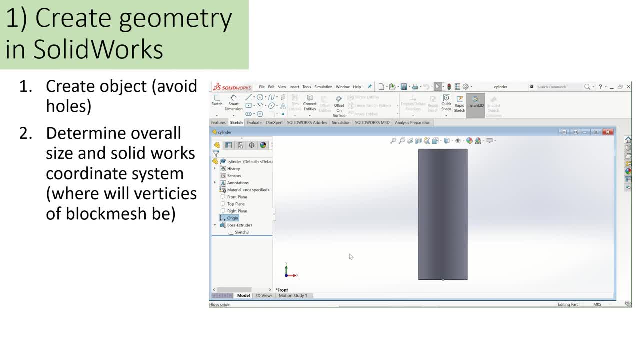 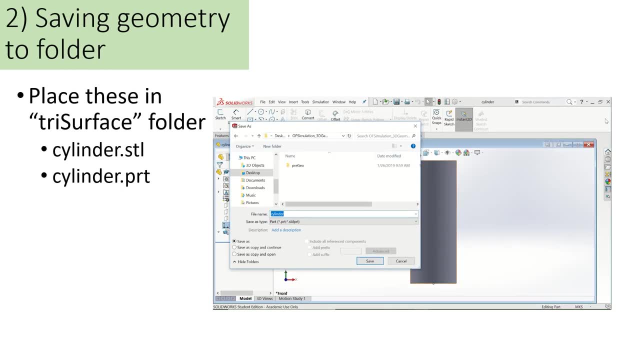 coordinate system which matches pretty nicely with the open foam coordinate system. and yeah, that's about it for the tips. So if you do decide to make your new geometry, the place you're going to want to save it is first off in SolidWorks. you go file save as. 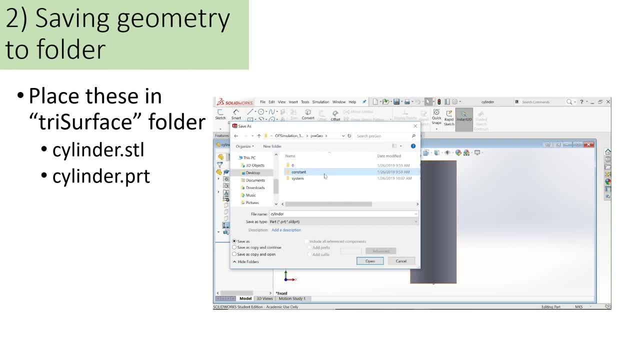 and then you go to file save as, and then you go to save as, and then you go to the pre geo folder, constant, and this new folder which isn't in other open foam simulations, it's called try surface, and you're gonna want to save your file in. 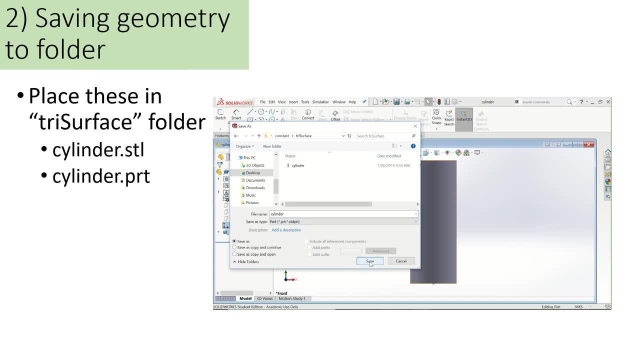 two ways in this folder. one is just as your regular SolidWorks part so you can go save and I would recommend using the same name cylinder just will make it easier later on in the tutorial. so once that saves, go save and just save and go on to the next page. 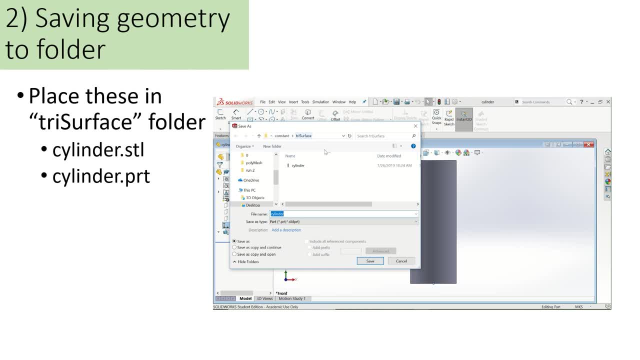 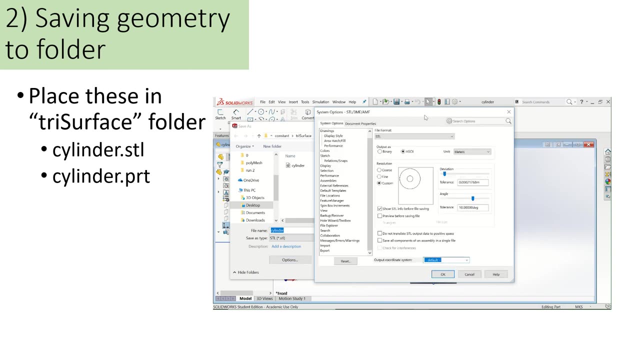 again file save as. and we're still in that tri-service folder. we're going to save it this time as an stl. so for your stl file you'll want to make sure that it's saving in ascii format. so that's good, press, ok, and then we'll also save it there. and we know it already exists. 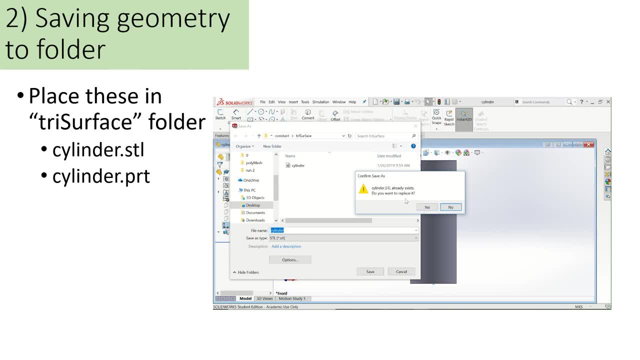 again. you can change the name if you want, but you're going to have to go through and change all the other names in, whether it's the like, the zero folders or elsewhere. so i'd recommend just keeping the name cylinder. even if it's not a cylinder, it's fine. 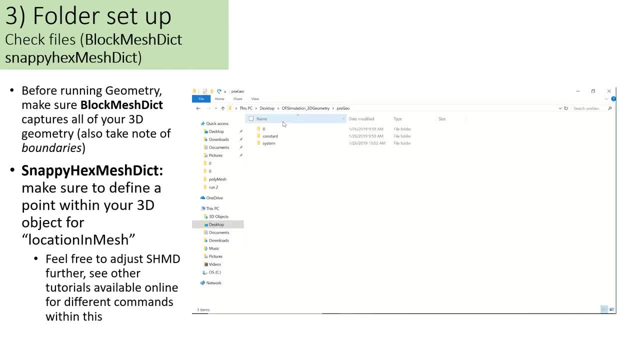 all right. so before we run our geometry we just want to double check a couple things in our folder um. so we just want to make sure that in the tri-service folder we have our two files. we have our 3d object file and our stl file, um. in addition, we want to make sure that our 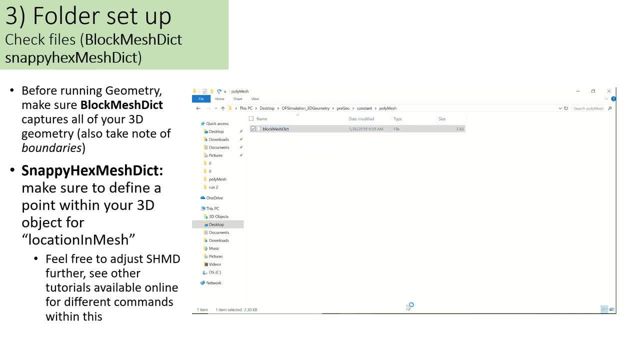 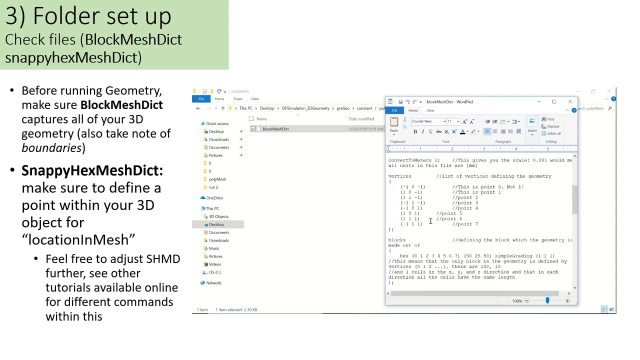 block mesh accurately captures this 3d object. so my cylinder is 15 centimeters in diameter and 40 centimeters tall, so in our block mesh everything's in meters and based on that, with these vertices, we should be able to accurately capture our 3d object. we'll also keep an eye and take a look at what our 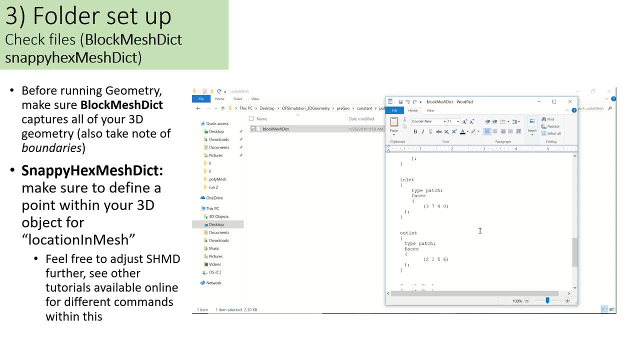 boundaries are. so i basically made an inlet, outlet, front and back and regular walls, so there's four walls and then an inlet and an outlet. so we'll be using those later in our boundary conditions. finally, we want to just double check in our system folder for snappy hex mesh. we want to both be able to see our 3d object. 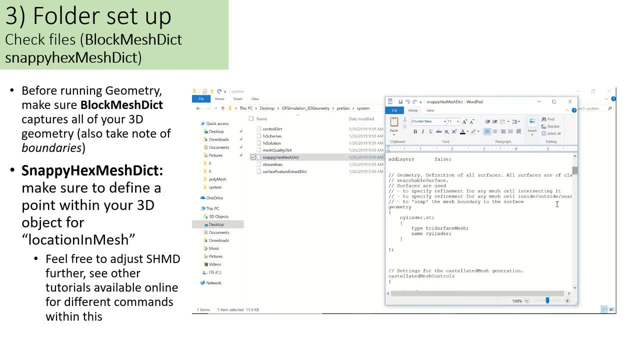 and our whole block mesh. so what you'll have to do is make sure that you define a point in mesh to make sure that this is a point that lives within your object and therefore you'll be able to see both of them when you accurately snap your uh do snappy hash mesh. all right, so it. 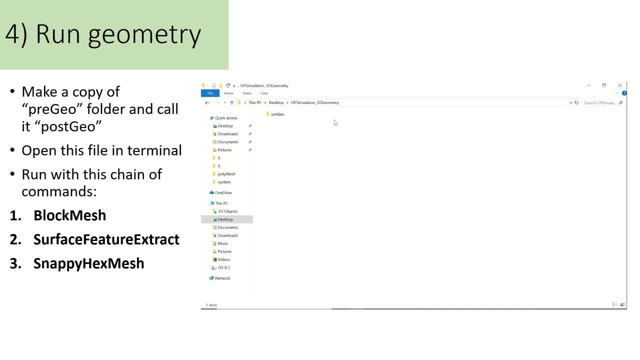 looks like we're ready to run our geometry, so that's pretty exciting. so what we're going to do first is we're going to make a copy of this pre-geo folder and we're just going to paste it right there, because we're actually going to run this bad boy. so next we're going to open this. open up this. 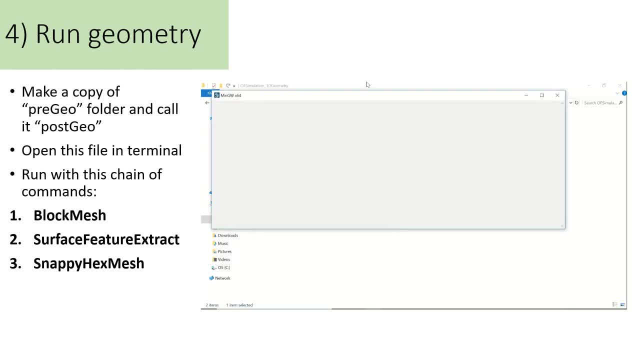 folder in terminal and you're going to use this chain of commands within terminal. so once it loads, you're going to run three different commands. the first one is just block mesh, so this is generating the actual block structure around our 3d object. next you're going to do: 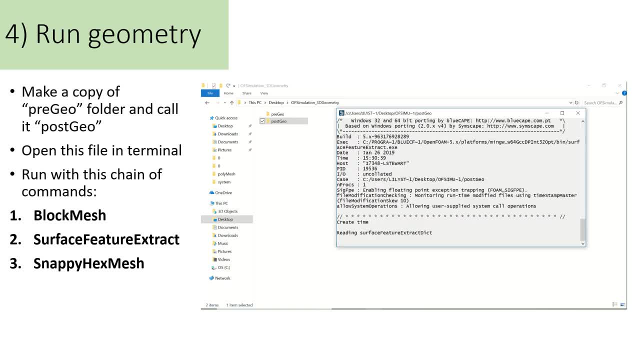 for surface feature extract, and so that's taking the surfaces off of our 3d object. and then, finally, you're going to use snappy hex mesh, and this one will take a little bit longer to run, um, but once we do that, we should be able to open it up paraform and see what we have. 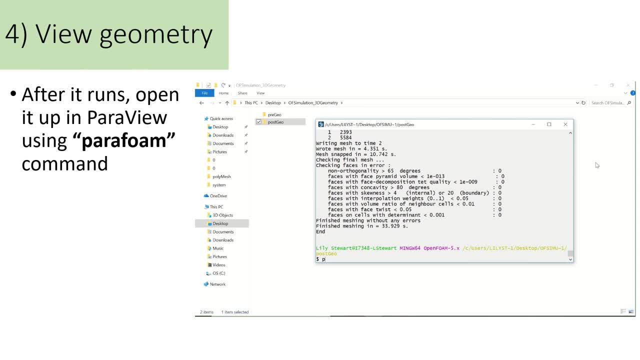 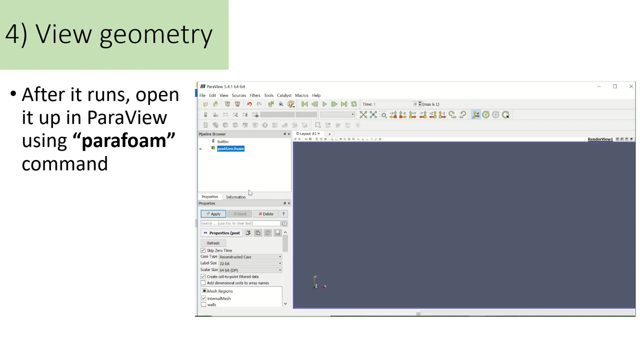 all right, so we are officially snapped. so it's time to open it up in paraform and see what we have. so it took us about 30 seconds to snap it, but it's not too bad, all right. so once we open it up in paraform, we're just going to go apply. 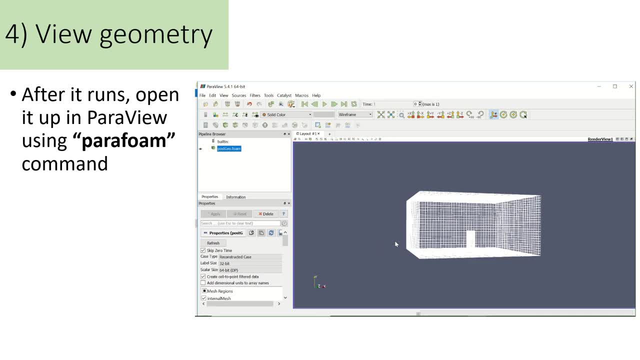 and then, to make it easier to see, we're going to go for the wireframe. so when we open up our 3d object, we're going to see that snappy hex mesh did a good job here. so we have our block mesh which is surrounding our object, and then we have our 3d object right. 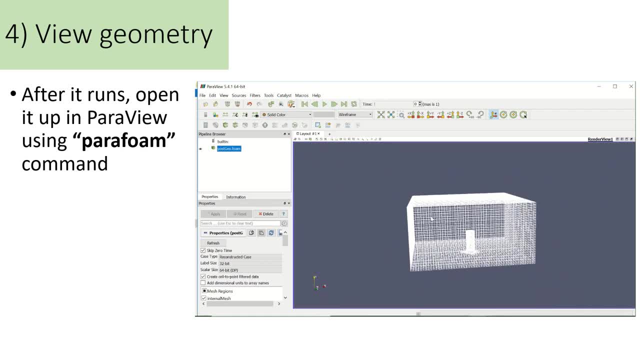 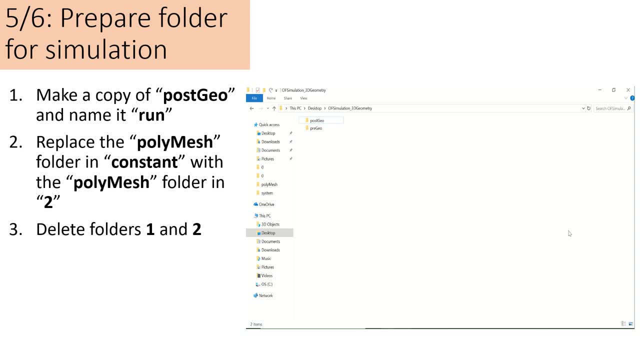 there sitting on the bottom of our box, just like we wanted. all right, so this next part, we're going to capture our geometry that we just snapped, but we're also going to prepare our folders so that we're actually ready to run our simulation. so the first step, what we're going to do, is we're going to take post geo, which has our snap geometry. 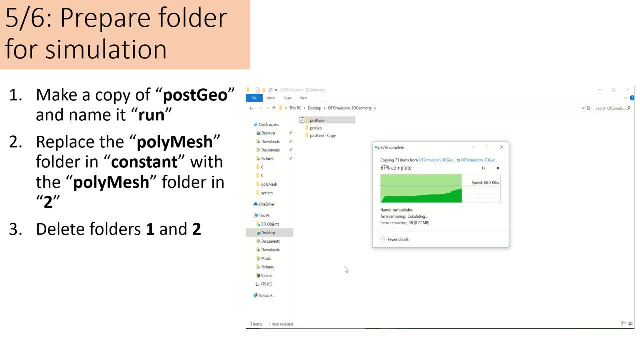 copy paste it right in this folder here, um, and then, once that's copy pasted, we're going to rename it. all right, so we're going to rename this folder and we're going to name it run, because this is the folder we're going to run later. all right, so within run, um, you see we have zero, one and two, so 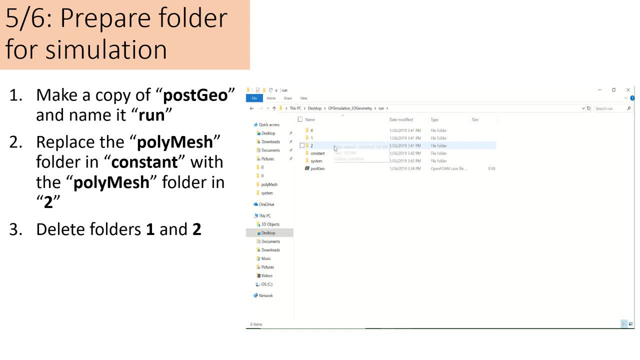 zero has initial conditions still. uh, one and two are like the snap: geometry is each iteration. so we're gonna do is we're gonna go into two. we're gonna take this poly mesh folder, so we're gonna copy that folder and we're going to delete this poly mesh folder in constant and replace it. 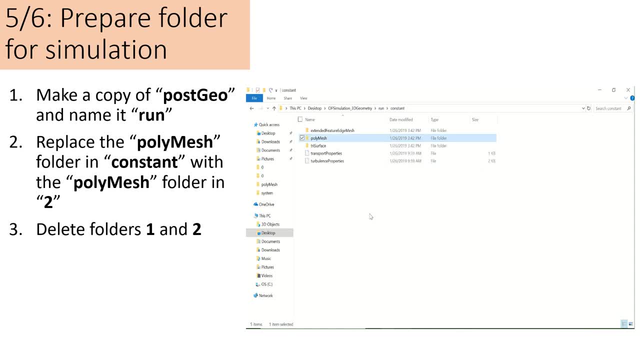 with that poly mesh folder from two. so you take the poly mesh from two and you replace the one in constant with that poly mesh folder. so now we have our snap geometry in our poly mesh. so now we're going to go back to our run, our overall folder, and we're going to delete folders one. 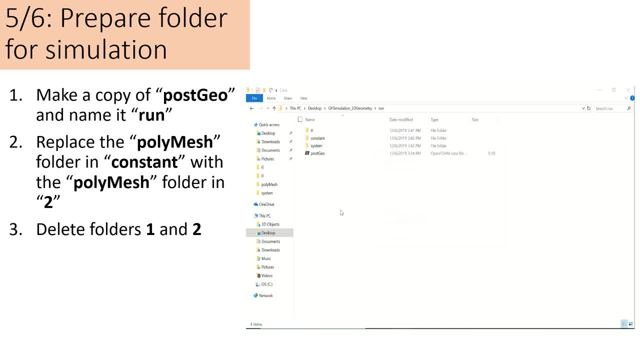 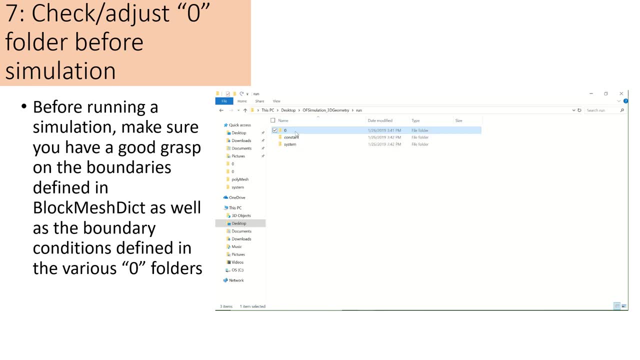 1 and 2.. All right, so now it's almost ready to run. All right, so before we run our simulation, we just want to double check our boundary conditions and maybe adjust them if we need to. So we're going to go into the run 0 folder- This is always a good idea, just to. 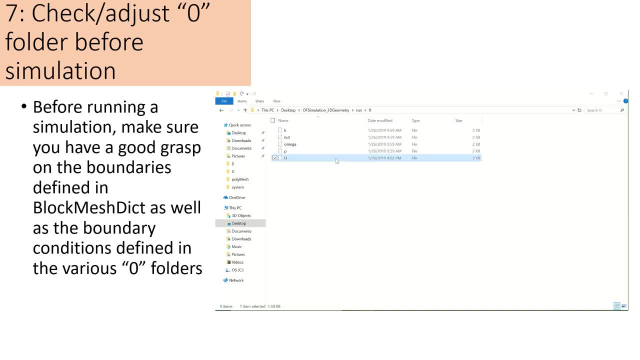 double check before you run, And also, so we're going to open up our U, which is velocity folder. So one thing I want to point out is, when you're using like a snapped 3D geometry, you're going to have to define an additional boundary, condition that wasn't in your original. 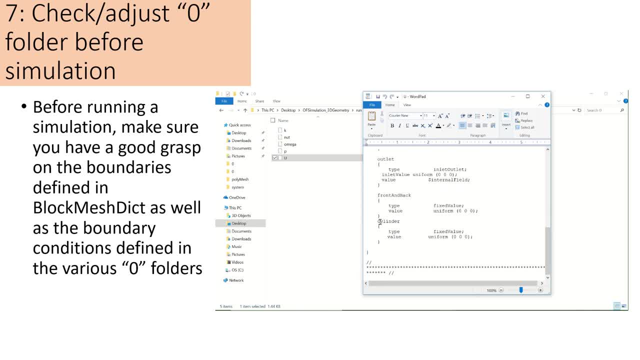 block mesh And that's going to be just whatever you named your file. So in our case we named it cylinder. That's why I had you name your 3D object cylinder earlier. It makes life a whole lot easier and you don't have to adjust a zillion files later on. So in our case we have cylinder as one of the 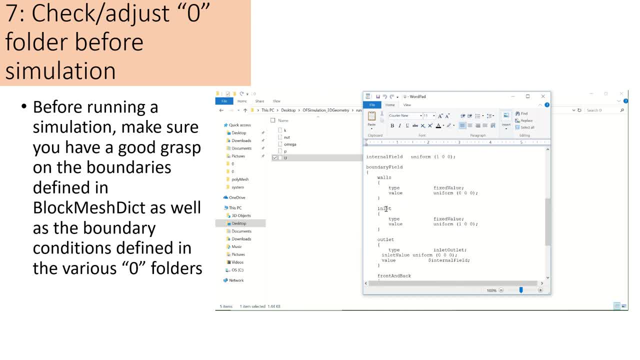 boundary conditions or boundary conditions, and then we have cylinder as one of the boundary conditions. So in our case we have cylinder as one of the boundary conditions or boundary conditions fields, and so anyway, so for the U file, for our little tutorial, we're gonna 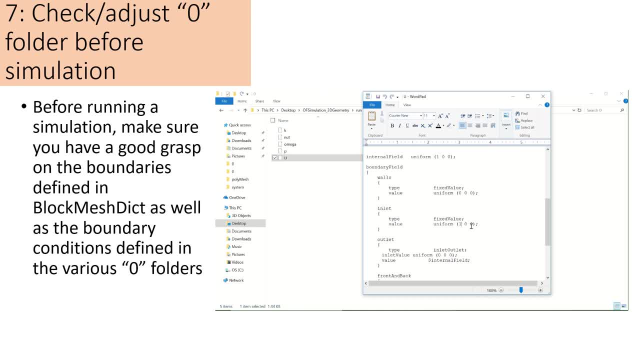 change this value at the inlet. instead of just one meter per second, we're gonna bump it up to five meters per second, so you don't have to do that, but it shows that you can easily go in and adjust before you run a simulation and if you. 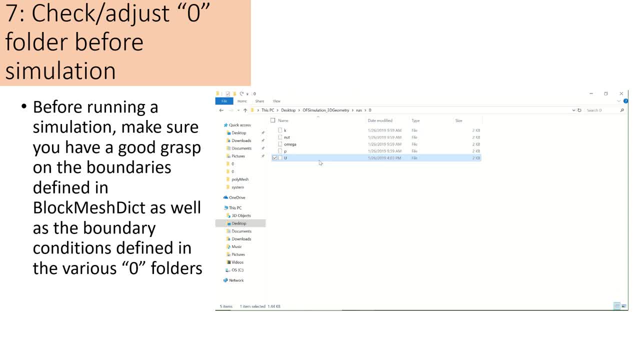 whoops. if you ever get confused about like what inlet outlet some of those boundary fields are, you can always go back. this is why we make so many folders. you can always go back to your pre geo folder, constant poly mesh into your block mesh dict and this will show you kind of explain further what you. 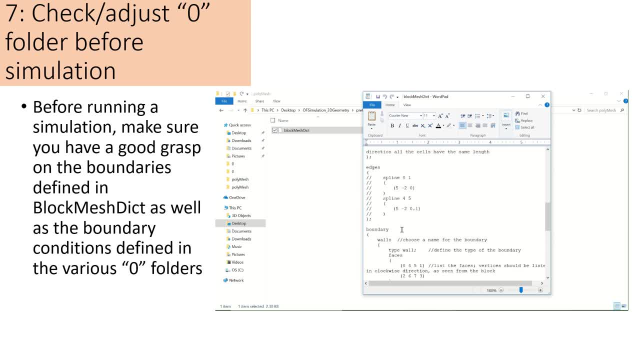 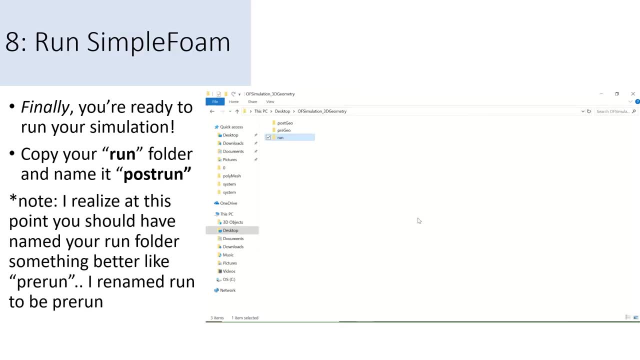 originally defined as your inlet, what you defined as your outlet, and it helps you visualize what's going on a little bit better at the boundaries if you get confused. all right, so I think now we're ready to rock. so we're gonna do is we're going to make a copy of our run folder and 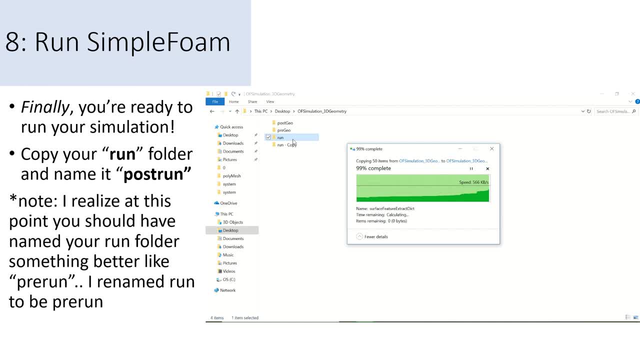 at this point you might want to name your original run folder something like pre run instead. we probably should have done that originally, but I didn't really think about it. so now we have a pre run folder and this one. we're not going to actually touch in terminal this run copy, though we're gonna name this guy post.